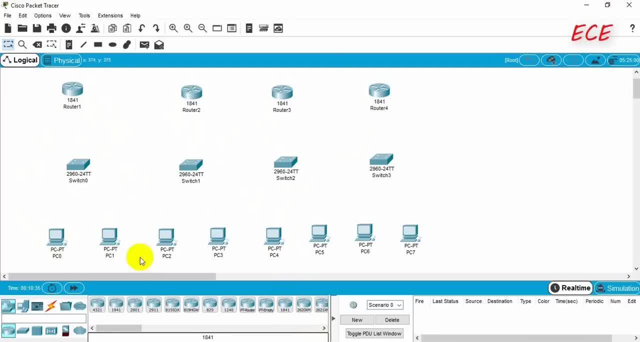 We cannot communicate with different network, with different IP address, using switch, So we need router for this. Let's connect them using copper straight thrower. Now we need to connect switches with the router and we are connecting first ethernet zero of every router. Now we need to connect the routers. 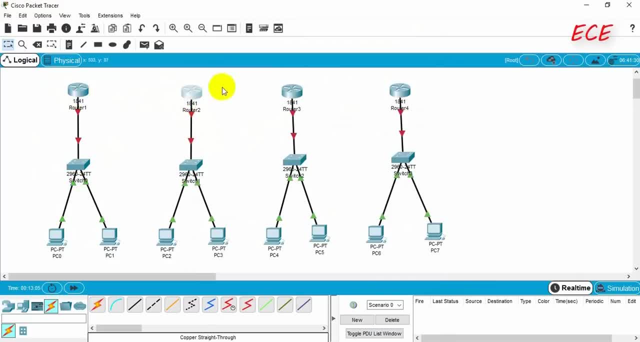 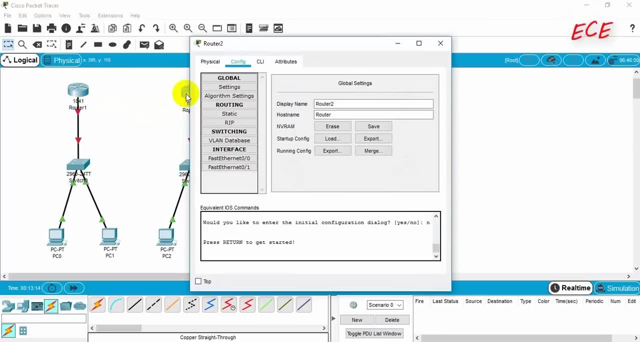 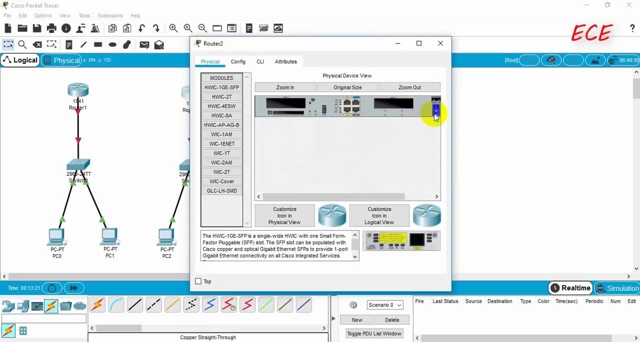 And you can see only two ports are here. One port is here, but there we need two more different ports For increasing the port number. we need to go to physical Turn off this switch. Then on the left side, go to WIC 2T. 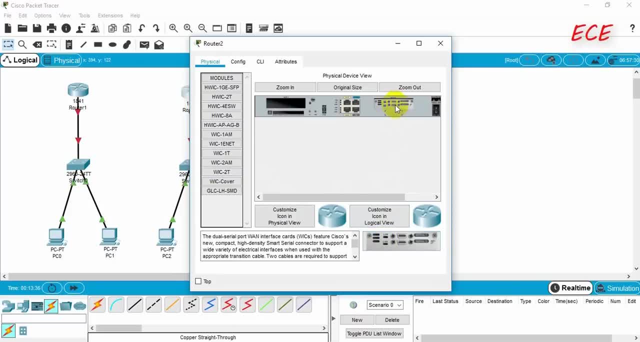 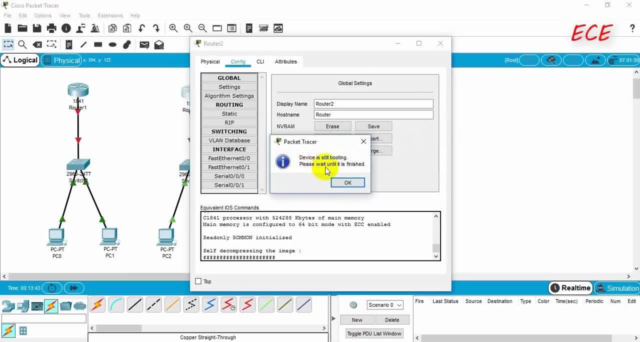 Then take this inside this box and turn on the switch. Now it is already. you can see that there are two more serial port here. We can use this serial port to connect the routers, So we need to do this for all the other routers too. 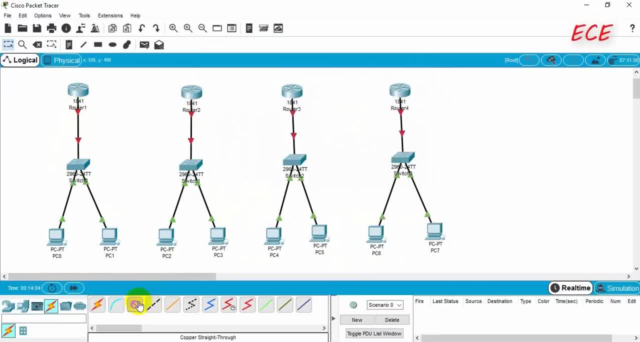 So we need to connect the routers. As you can see that we cannot connect ethernet with serial port, So we need to have serial port in other routers too If we want to connect them. So let's do the same thing again. Go to configuration. 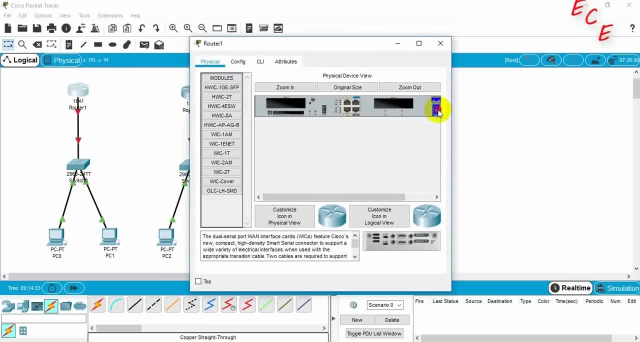 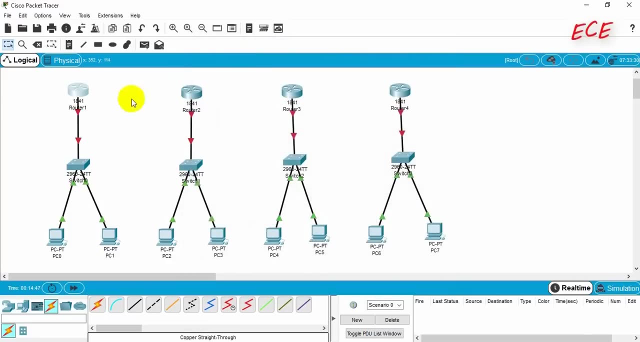 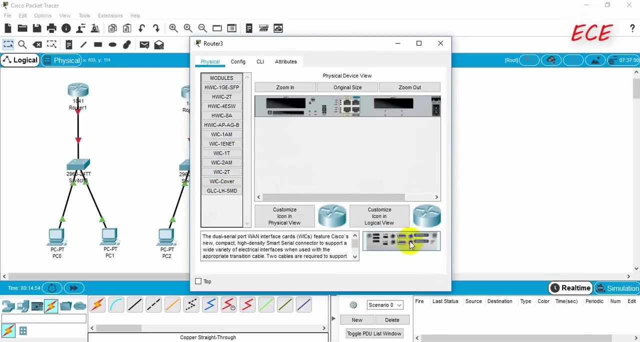 You see there are only two port. Turn off the switch and go to WIC 2T and take them in that box and turn on the switch, Wait for the system to boot and then do the same thing for other routers too. Now our system has booted. 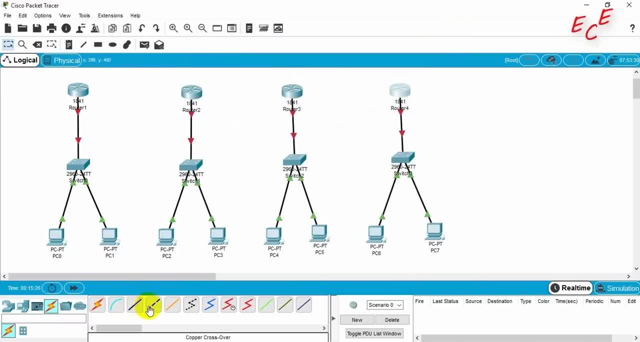 It has completed the booting And it was fast. We can now connect it. So let's connect the router. You will connect with serial data, With serial port 0.. With serial port zero And with serial port 2.. then serial port 1 with this router, serial port 0. 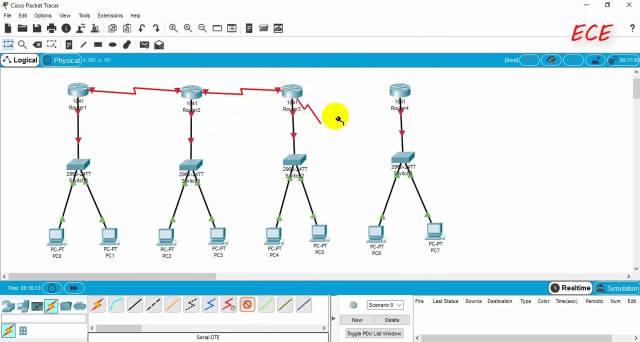 and this one's serial port 1 to the last one's serial port 0 0 0. now we will take some notes here. the IP address, the PC's IP address, will be always different. only the two of them will have same IP address, with the host ID different here. 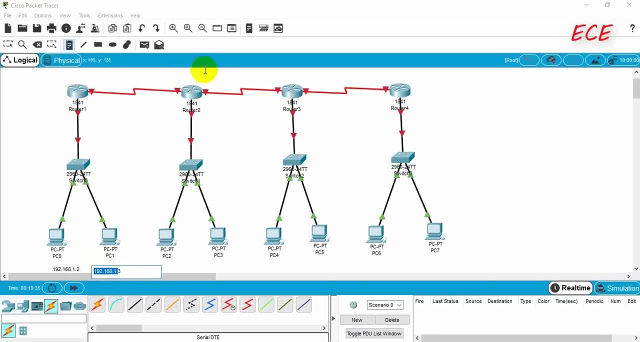 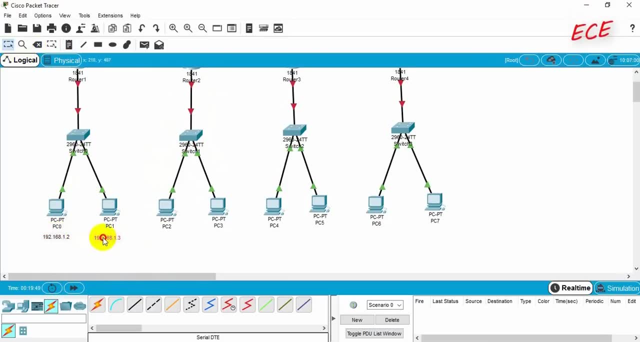 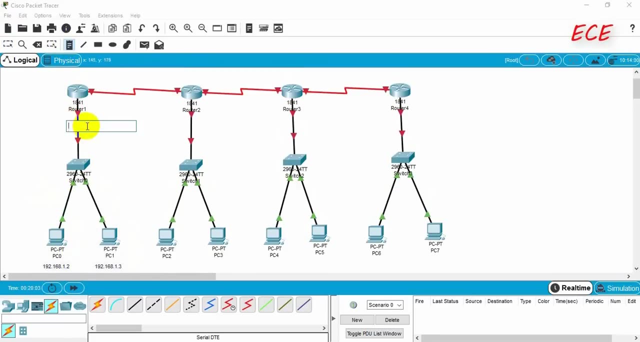 you can see that the IP address is 192.168.1.2 and .1.3, so we will always take the host ID as 2 and 3. only the net ID will be changed and here inside the router and switch connection, this will be .1. 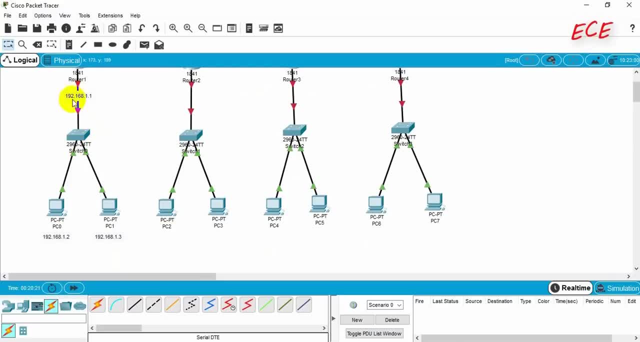 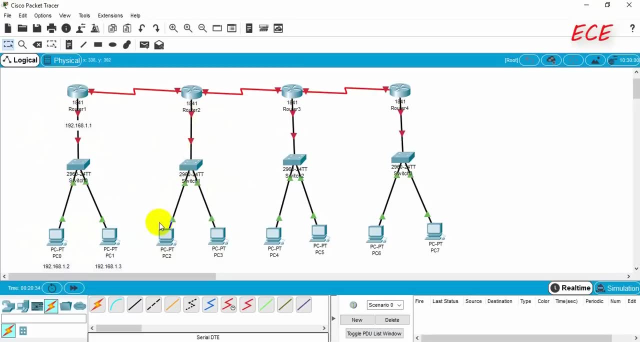 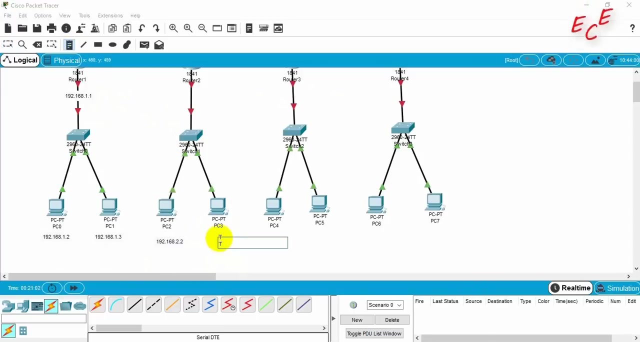 we will make the other network like this, so that we don't forget the connection. this one will be 192.168.2.2, so the IP address is different. you can see the net idea is changed and now among this two, from the same IP address, only the host. 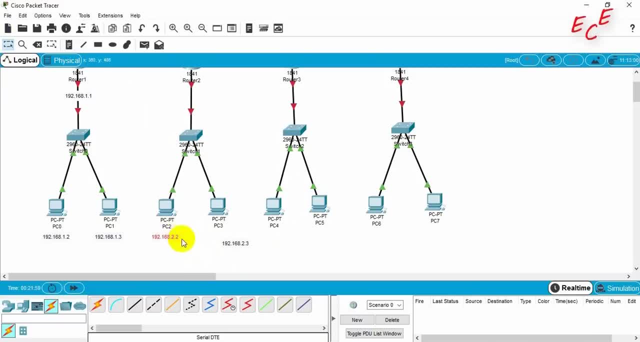 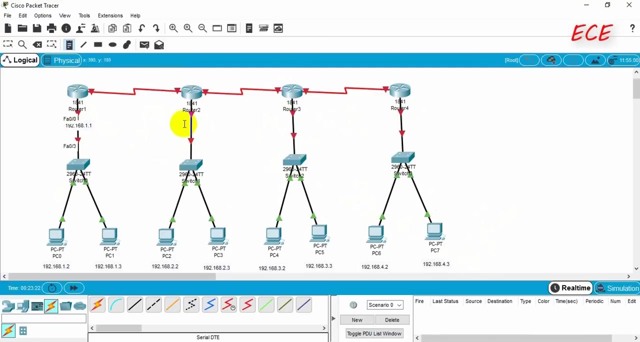 ID will be different. Thank you, And now we need to give the IP address for this root 2.. This will be 2.1.. And the next one will be 3.1.. And the next one will be 1.1.. 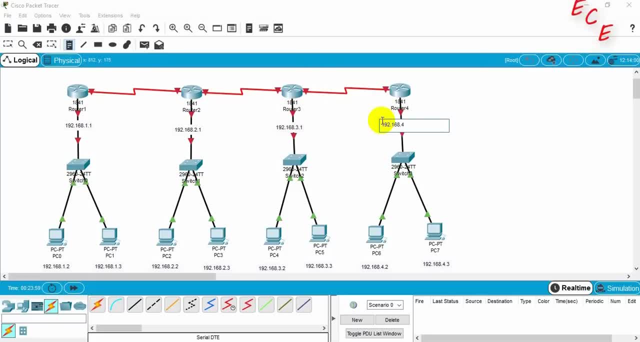 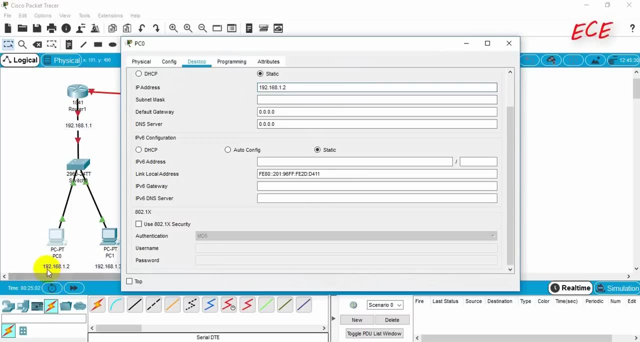 And the next one will be 22.168.4.1.. Now we need to set the IP for the PCs, to go to desktop and IP configuration. Here we need to write the same IP address we wrote in the note And we need to change the gateway letter. 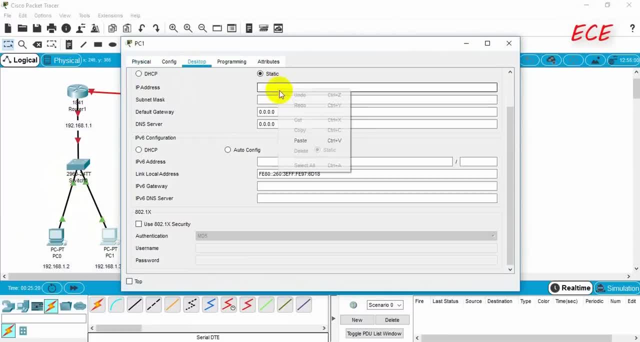 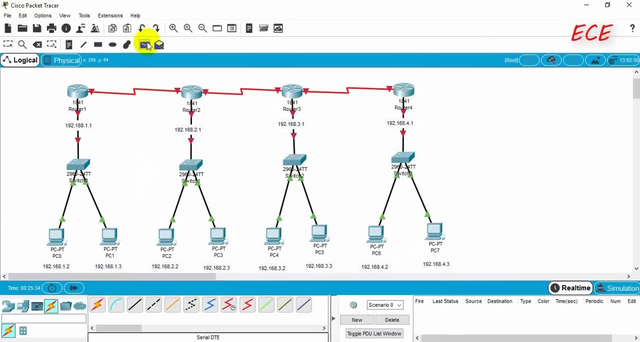 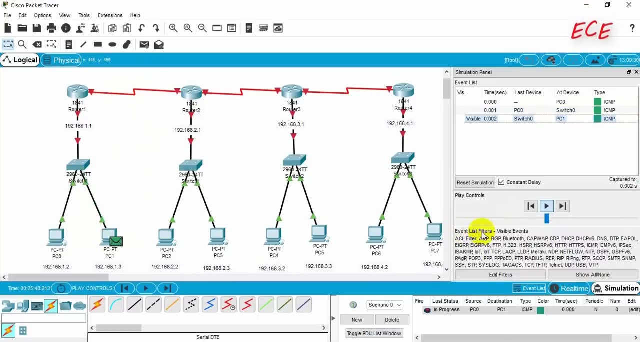 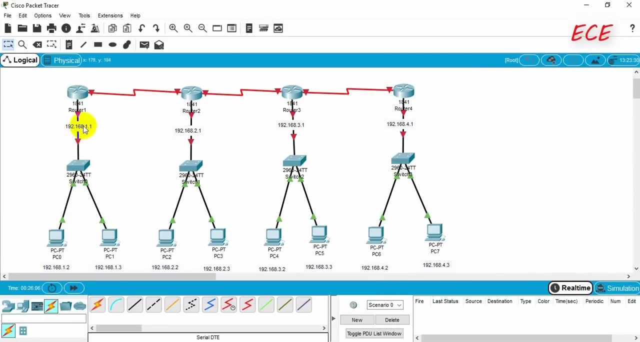 For now, we will just set the IP address and check if this is working. Now, if we send message from PC0 to PC1, you will see that it is working properly. Process will be successful Here. we need to give the gateway and gateway will be 0.1. 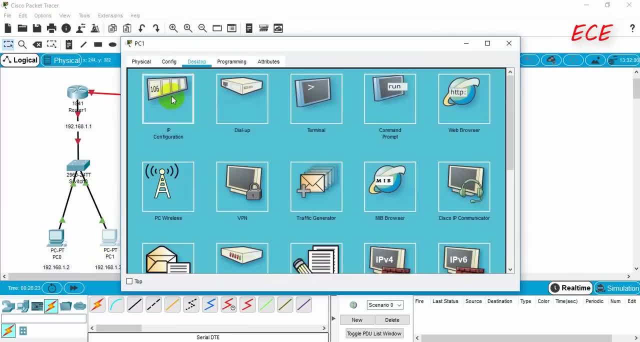 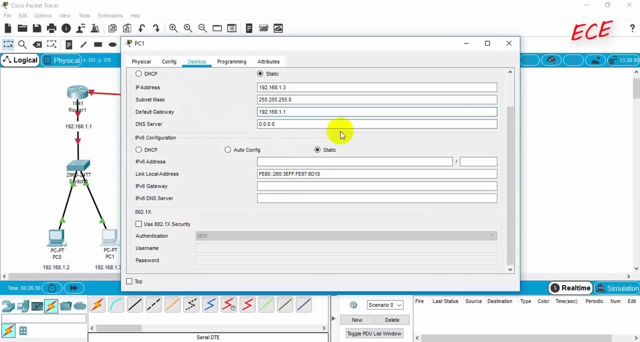 And the IP address from switch to router, And both PC2 and PC3 will have the same gateway. So we are using the same default gateway for both the PC, And now this one's IP address is .2.2.. And then the gateway will be .2.1.. 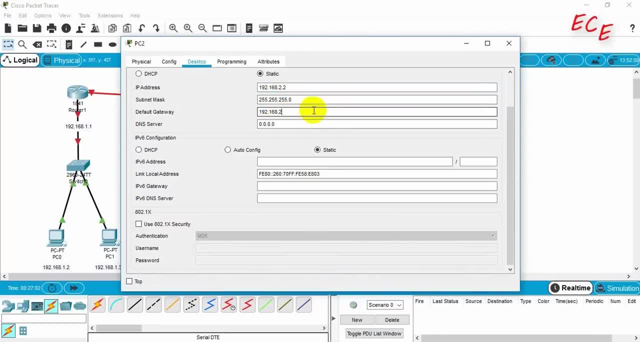 Because this is a different network. the IP address will be different, The net ID is different. Then this one: Here it will be 0.2.1.. Here it will be 0.2.3.. And the gateway will be 0.2.1.. 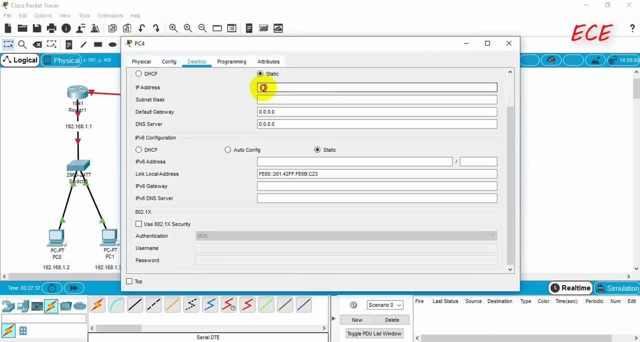 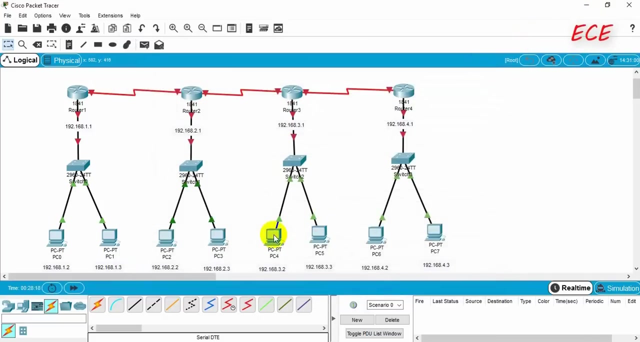 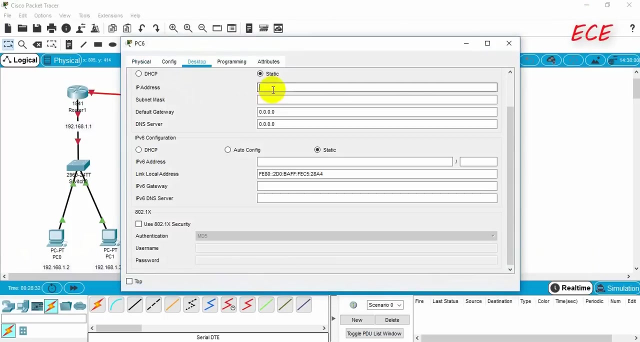 Then this PC. This is 3.2.. And here, 3.1. The gateway is the IP address between the switch and the router. The gateway is the IP address between the switch and the router. Remember that. 4.2.. 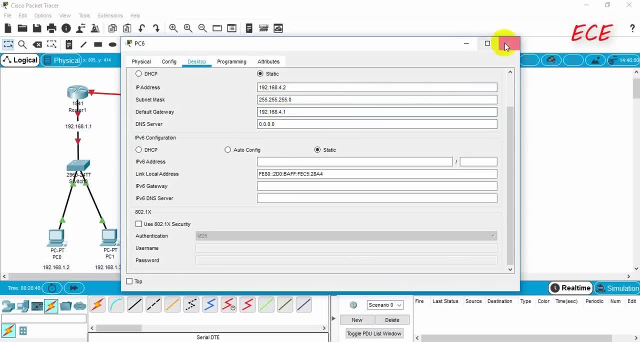 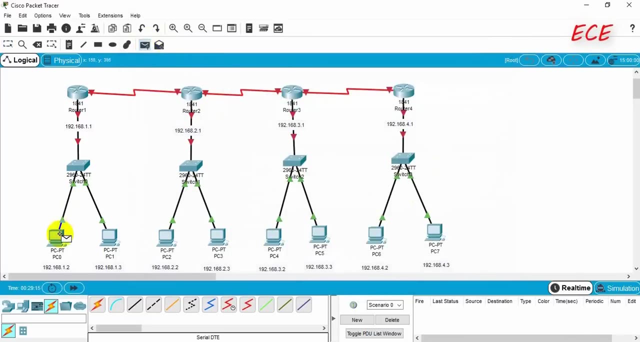 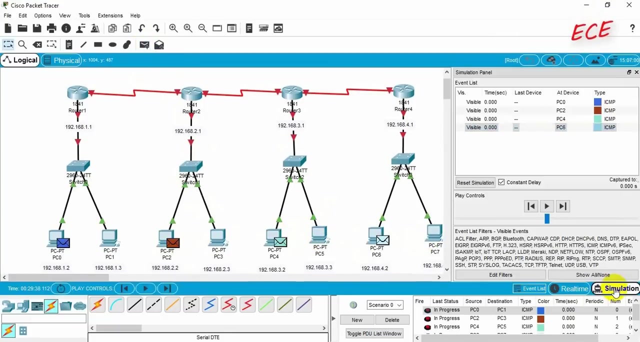 And the gateway will be 4.1.. Now if we send the message from every PC in the same network, you will see all the process will run properly. We will see all of the processes will run properly. Now, if we want to send message to the back end: прорamps. 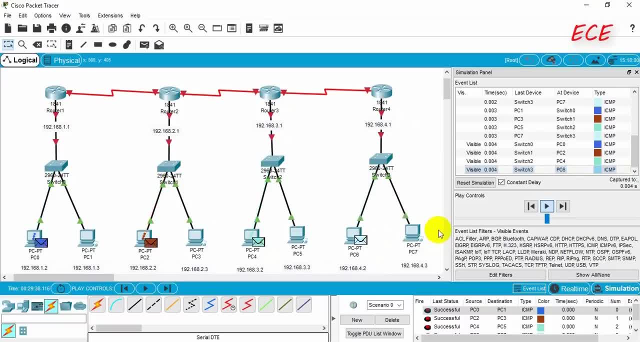 Therefore we will need some 24 hours to decode all the IP addresses, But right now, if we want to send a message from main PC, we will need 4.2.1.. Ok, so we are using the same network, So we can go directly to find out the adapter. 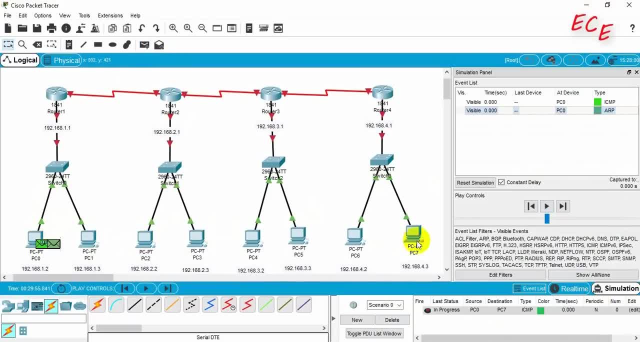 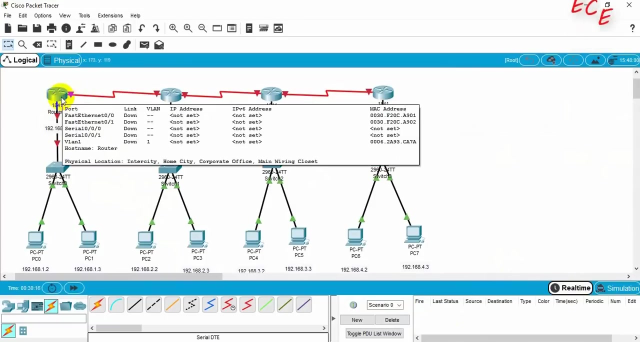 But now want to send message from a different network to another different network, you will see that the message will not reach the router because we did not set the IP address in the router. we need to configure router to. you can see the process. status is failed. so now we need to work on the router. here we did not. 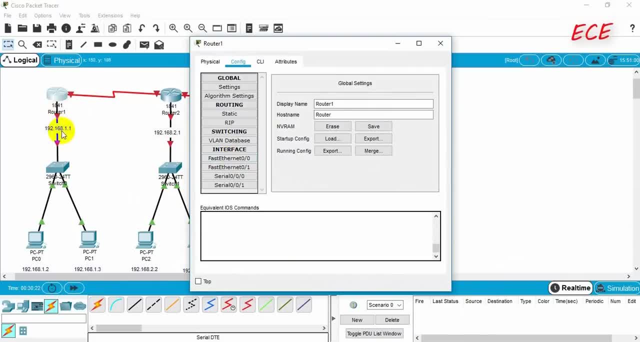 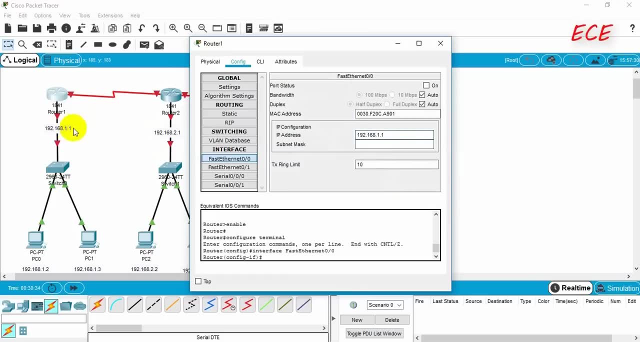 set any port yet. so let's go to first 800 0. this line is first 800 0. so here we need to give the IP address of this line, that is dot 1, dot 1, then the subnet mask and turn it on. you can see the green mark for this line. and now we 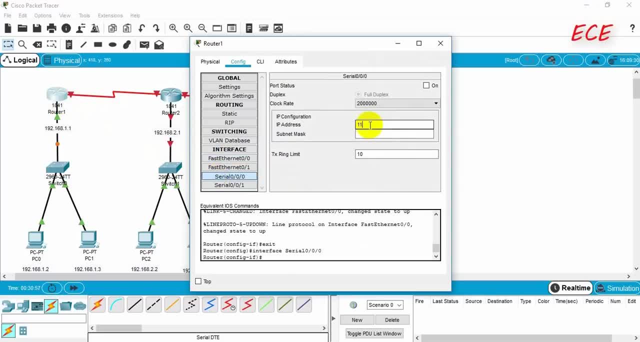 need to give serial dot 0, 0 here. let's set a class, a IP address that will be 11 dot 0, dot 0, dot 1, or we can set it to. you can set any IP address here. we are taking class a for this route and all. 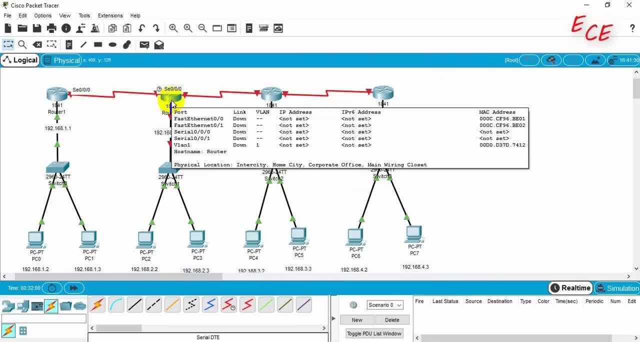 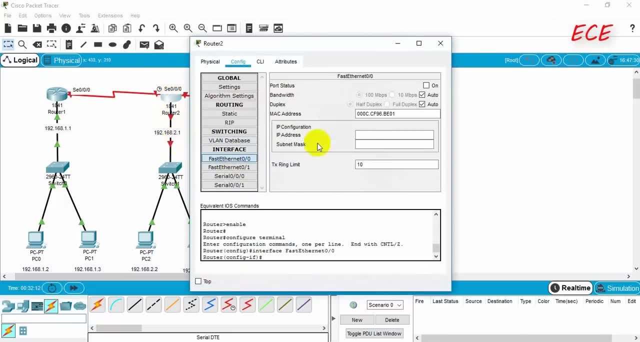 the other network was class C IP address till now, and here first 800, 0 was this line. so we need to write 192, 168, dot 2, dot 1. this is the IP address for Ethernet 0. and then we did not connect anything with first 800 0, 1, so we will go to the 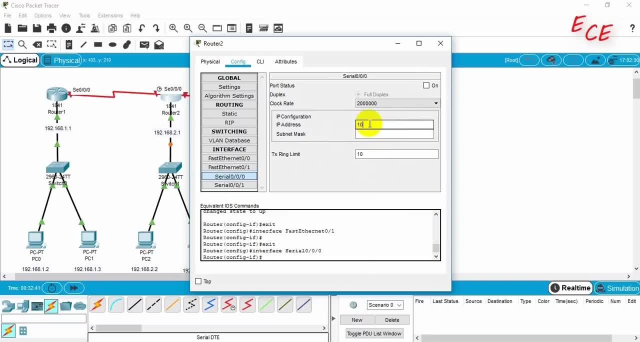 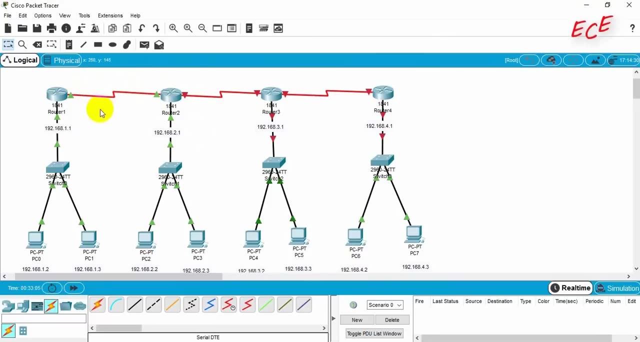 serial connection. here. serial dot 0 was connected with this route and that will be 11: dot 0, dot 0, dot 3. let's say you can give any host ID but the net ID will be 11 because we need to have the same IP address for a same route. 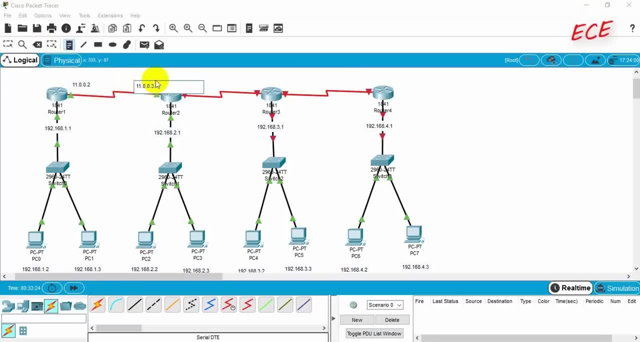 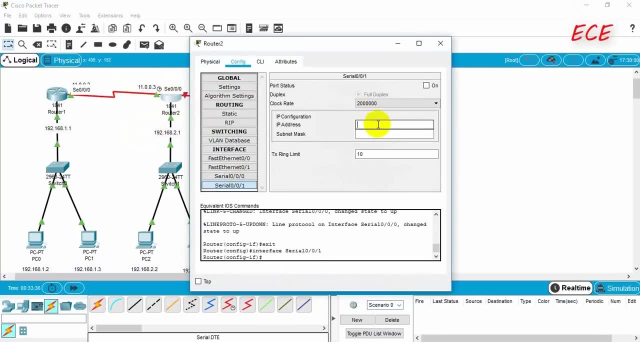 with the other port 0 & friends connect to you. shaken 0 dot 0, 0 dot 3, and now we need to connect this side too. so let's go to serial dot 1 and here, if we want to write it like this, you will see that we cannot write it. we need to have. 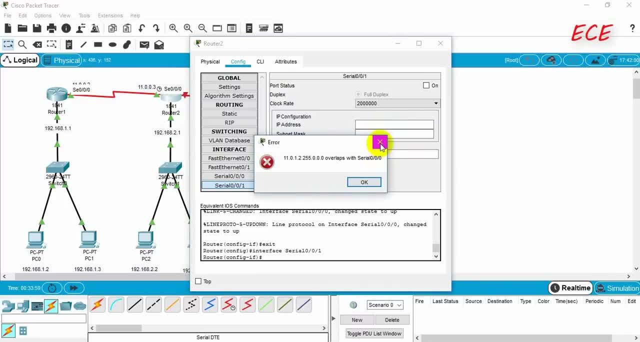 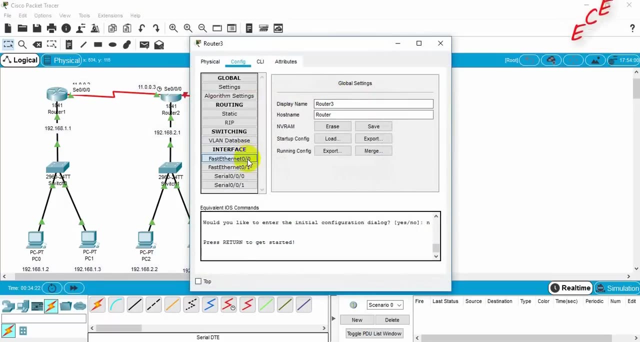 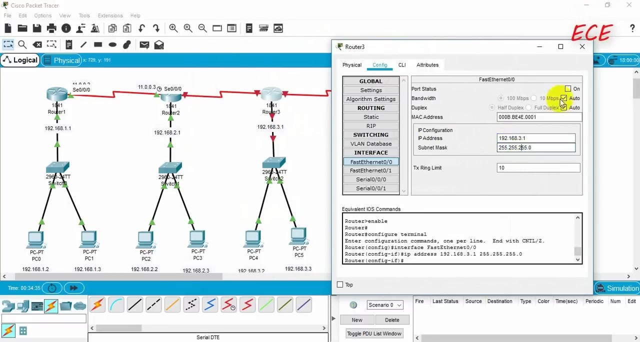 different IP address for this site. to even change the host ID, it will not work. it will overlap with the cereal port 0. so we will go like this and turn it on. and now the next router. for the first Ethernet 0. this was our IP address, class C IP address- and for serial port 0: it. 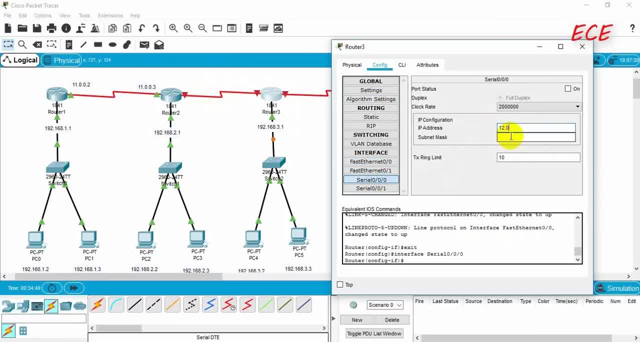 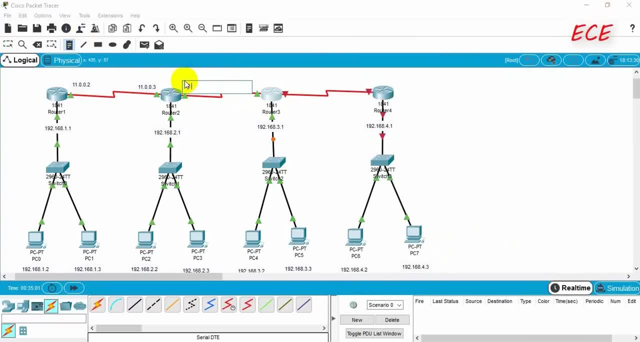 was this site. so we need to write 12.0.0.3. and now you can see that this route is also green. let's write it down. I'm maintaining a similar pattern here so that we can write the network easily later. so all of the host ID is 2 and 3 and the net ID will be. 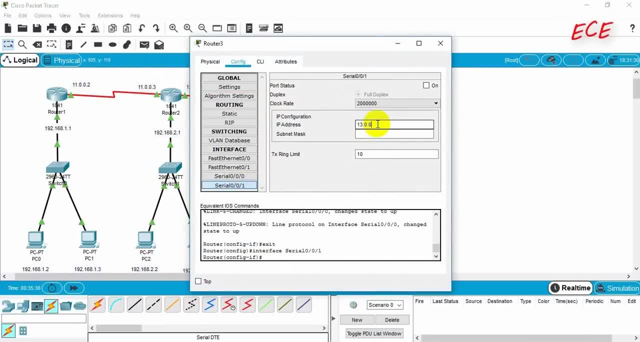 different, and the next one will be 13.0.0.2 and the last one. we need to connect this one too. first, Ethernet 0 was this one 4.1, and the serial port 0 was connected to the third router, so we need to write it like this: 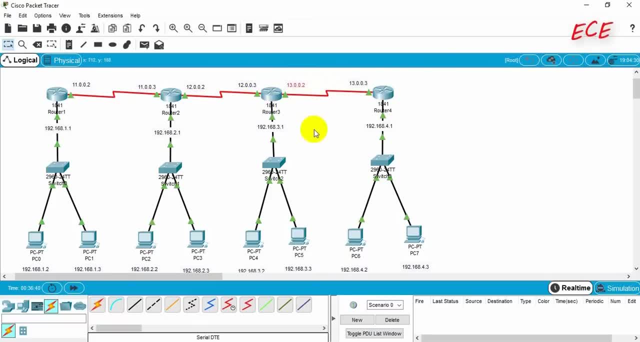 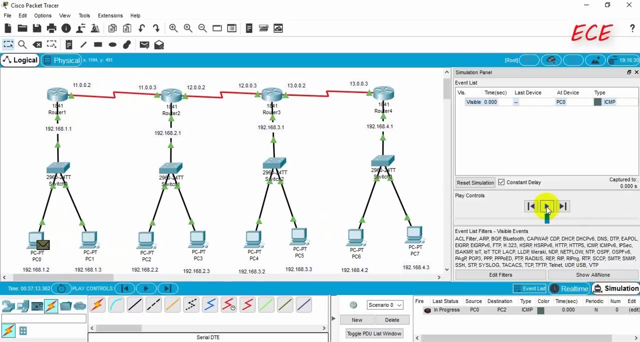 now. we just wrote all of their IP address. but if we want to send message, we cannot send the message till now because we did not define any of the network: from where the data can go to which road. we need to define that too. if we see, now you can. 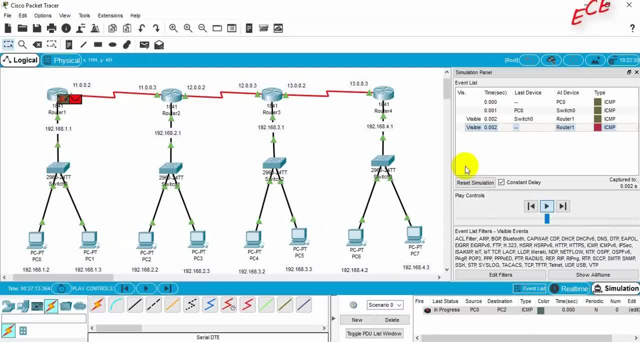 see, the data will be returned back from the router 1 because router 1 does not know from this port where they need to send the data to. and now we can see that now because we did not define any of the network from where the data can go to. 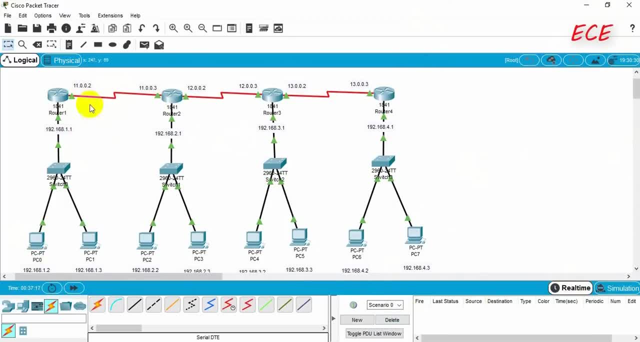 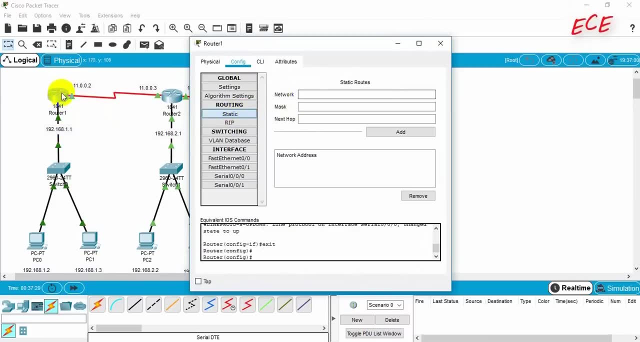 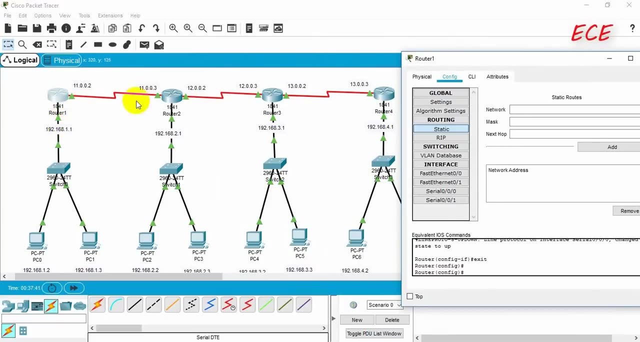 need to send the data. so for that we need to define the network here. so for that let's go to routing and then static. here we need to write the network name. from this router we can go to the second router. from these two pc, pc0 and pc1, we can send data to second router, third router and fourth. 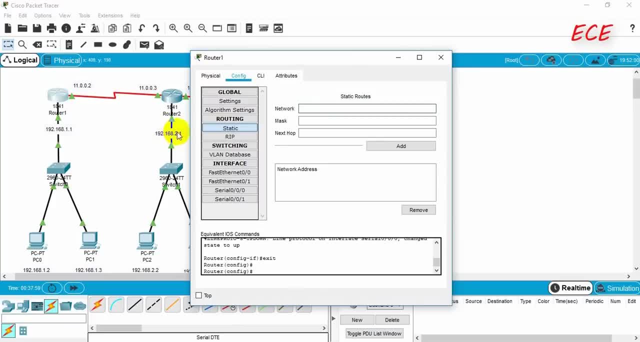 router. so we need to give all the network here one by one. so first let's go to the second router. so from the first router the data will be sent to second router. so second router will be all the network with the net id 2.0. if we write dot 0 then it will mean all the network with 192 168.2. 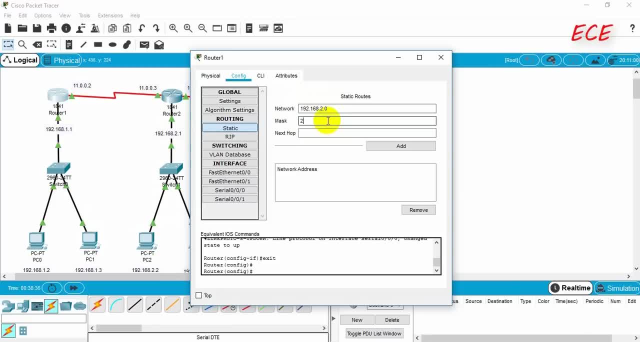 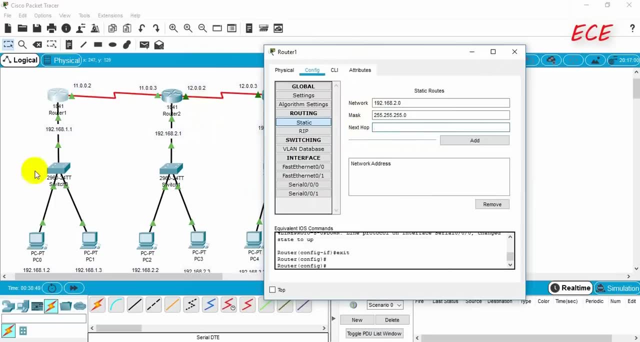 in this net id. we can use any host id because we are using dot 0 here in the network. and then the mask id was class 3 mask id because it was a class 3 ip address. so we need to write the subnet mask like that: 255, 255.255.0. 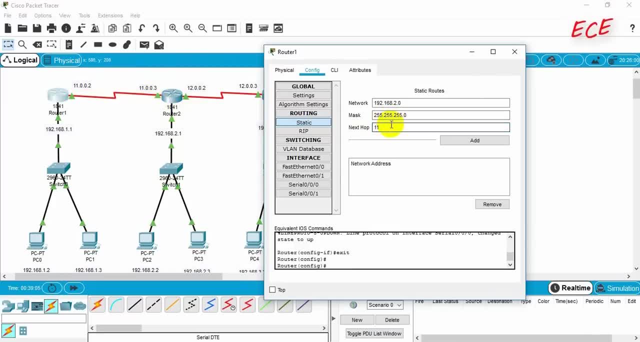 and the next hop. the next hop is actually the ip address near the next router. so here the second router's ip address was 11.0.0.3 and here the net. if we add it. you can see it was already added. so now here we need to specify. 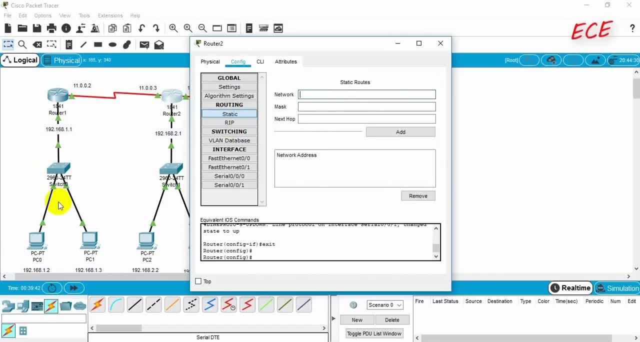 this network in the second router because the pc will send back a signal to let the first pc to know that it has received the data. so we need to write the same for this network 2. this was 1.0, so all the id from 192 168.1 will be accessed via this. and here the next hop will be the first router's ip address. we are accessing from router 2, so we are right here. the address is 192 168.1.0.2. we are accessing from router 2, so we are like the first routers IP address as next hop. So now, if we send from PC0 to 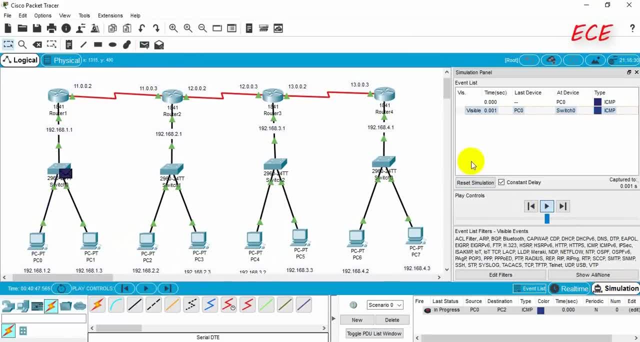 PC2, you will see the data will be sent properly and the process will be successful. Now you can see the data is passed from router 1 to router 2 and it is sent to router 2 and it will send back a signal. so 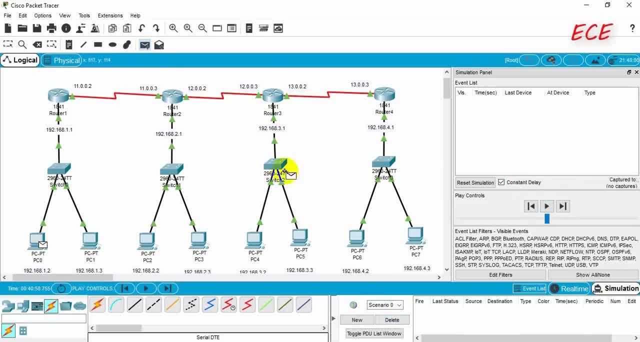 okay, now you can see successful. but if we want to send any other router, it will not go in that way. You will see that data will return back from the router 1 because router 1 does not know how to reach PC4. because we did not give the 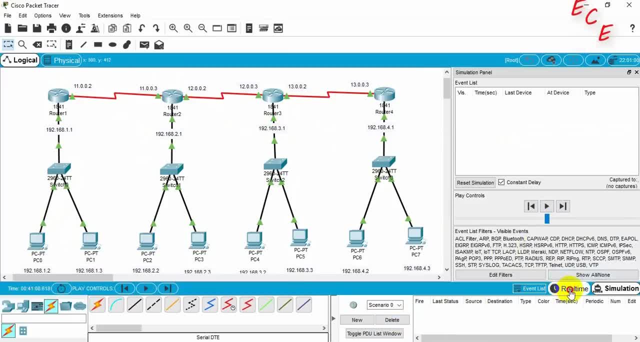 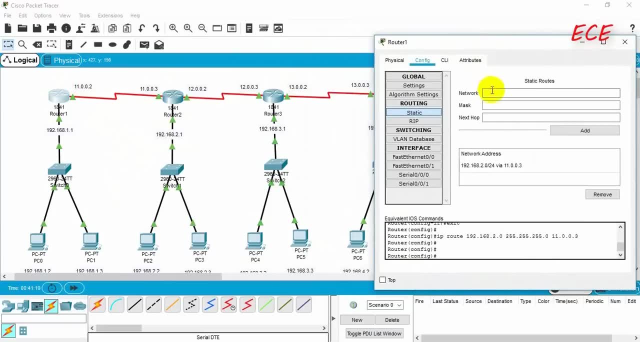 network in the any network of the router. so let's go back again in the static and let's add the other network too. like we have added here, we need to add the next hop properly in this case here. first, the network will be 3.0. 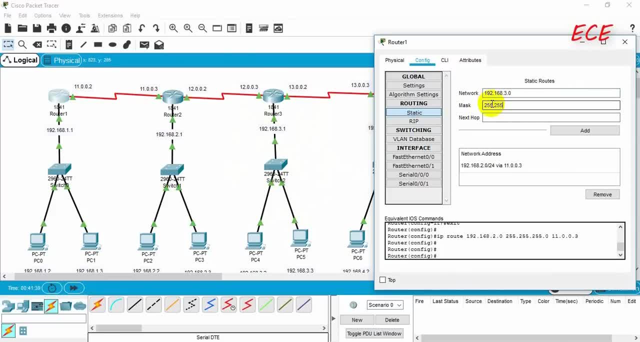 for this whole network, and here the mask will be as always. and here the next hop for accessing this network. we need to go from this, this route, so here to here, and we need to use this route. so this will be our next hop. we cannot just send the data from router 1 to router 3. we need to pass it. 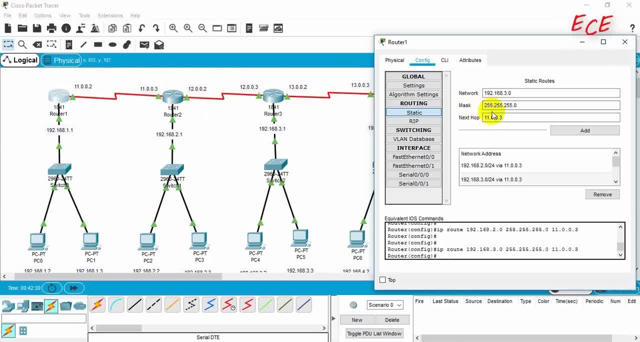 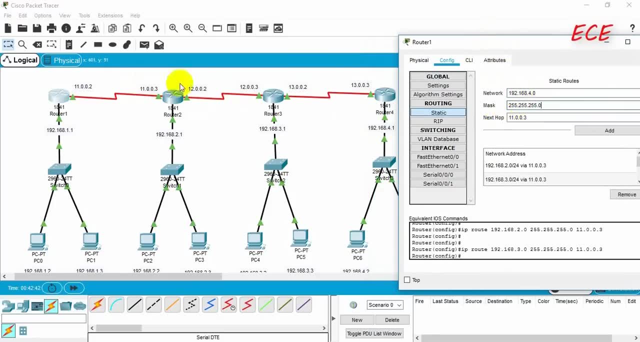 from using this route only. so we are using that data and here, if we want to use this network, so we need to write you 4.0 and the next hop will be same again. we need to use this route only. we cannot send it flying from router 1 to router 4. we added all the main network and now we need to add the network between. 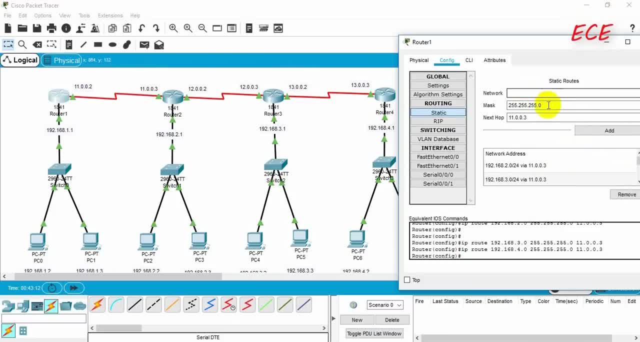 the roads. so let's just delete this and see this properly, because we will use the same route for every other router too. here we need to access this route through the first route. so 12.0.0- all the network from this route will be, and here the next hop will be 11.0.0, 11.0.0.3. 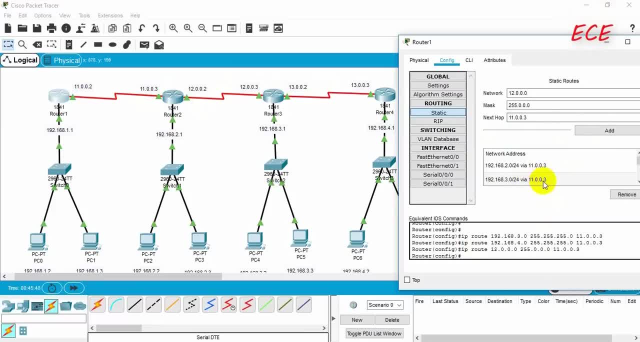 so now we are accessing the second route through the first route here. okay, now we need to send data from router 1 to router 4.. So we need to access route 3 using route 12.. I'm using road to make it easier to understand. So 3.0.0. here we will. 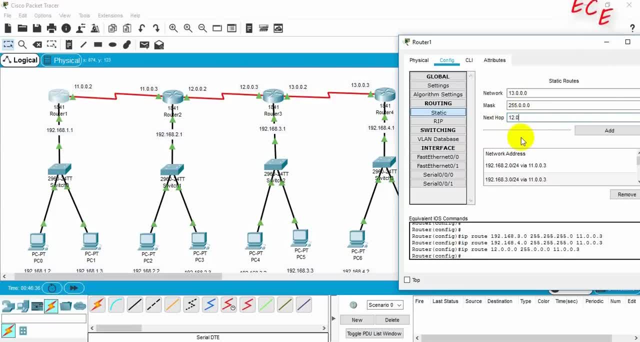 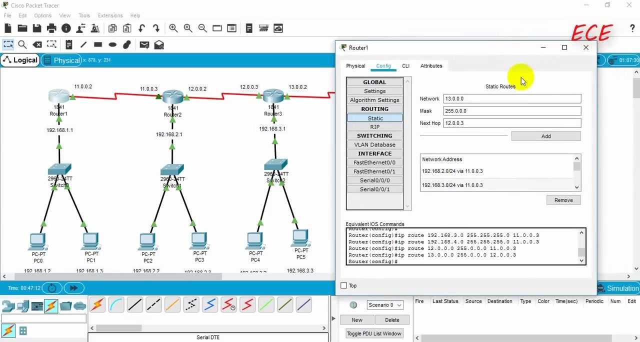 access this route, but we will access it using route 12.. So here we are accessing route 12 using route 11 and then accessing route 13 using route 12.. So by using this, we can access all the network. So now, like this, we need to add network in all the other routers too, one by one. 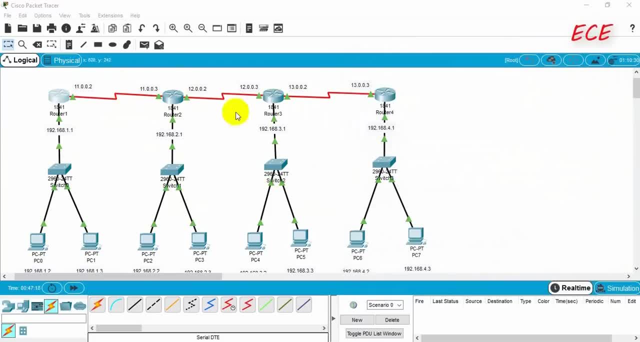 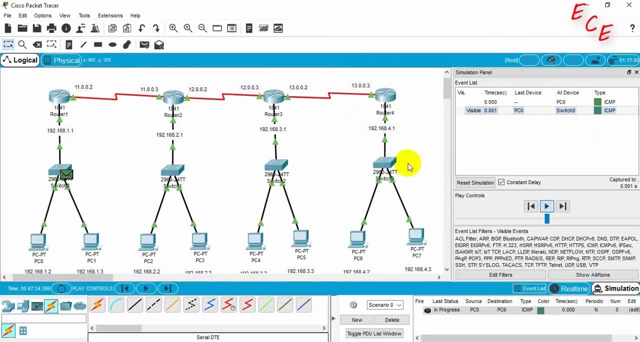 We need to do this properly so that the data reach them. So now, if we want to send data from here to here, you will see the data will go, but the signal will not get back here, so the process will fail. The data will be actually back from the second router because we have 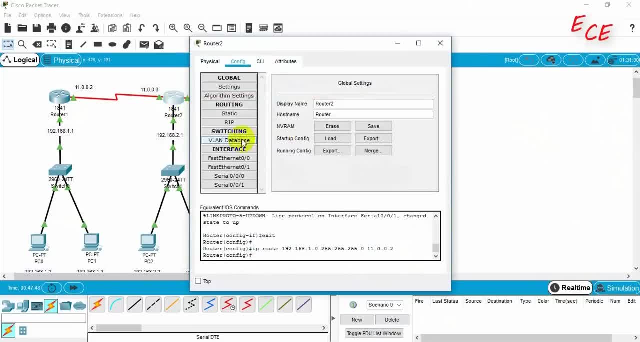 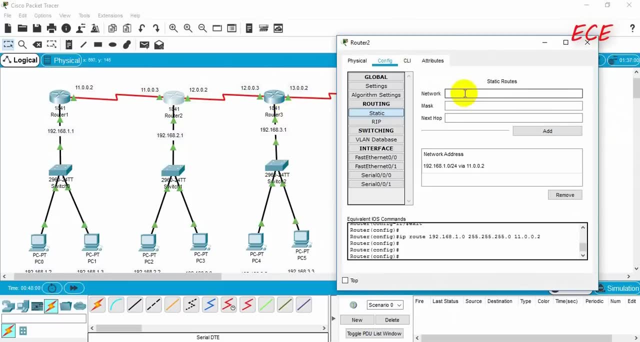 we have configured the second router a bit, but not the other router, so we need to add the other network too. So from second router we actually added the network for first router, but third and fourth router we did not add it, so we need to add them. So it will be 3.0 and the mask will be. 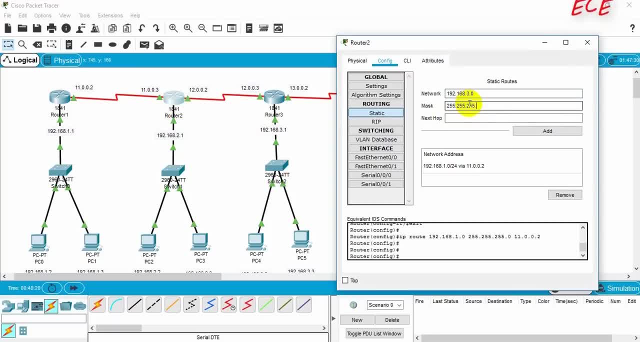 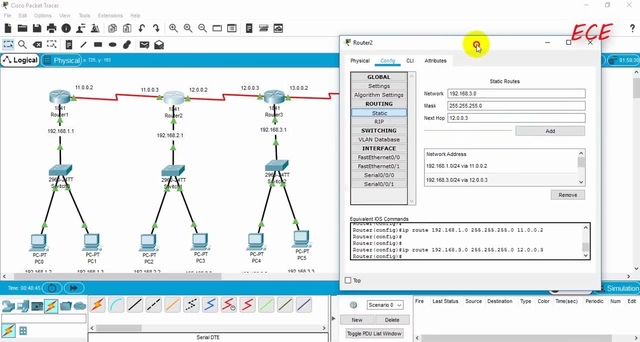 class 3- sorry, class C- IP address. so like this. and then the next hop will be: we want to access the router 3, so we need to add the router 3's IP address, 12.0.0.3, and then add it. Now we need to send data from router 2 to router 4.. So 4.0. 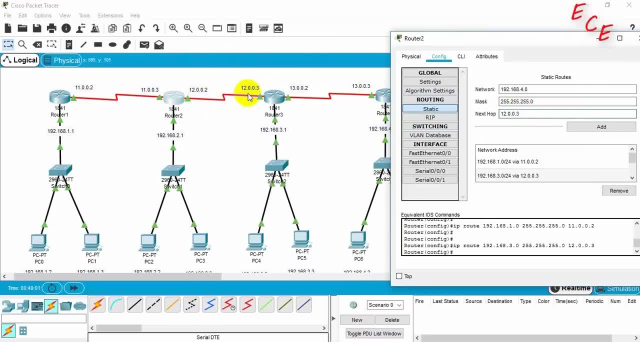 and the next hop will be again the same. we need to access it through this route only. we cannot jump over one. empezar at this спас. So in this last phase the thing is 40ら bakey and begins to add 8: mobility И not primary難い Kоль. The next stage is doing all the actions needed to do the previous tasks for the home office and customers, right down the radar. all the peuples are present and all来了 and seizing data from the hecho queve the sections of the front end of the interface. No problem, No, there is measurement at the front end. 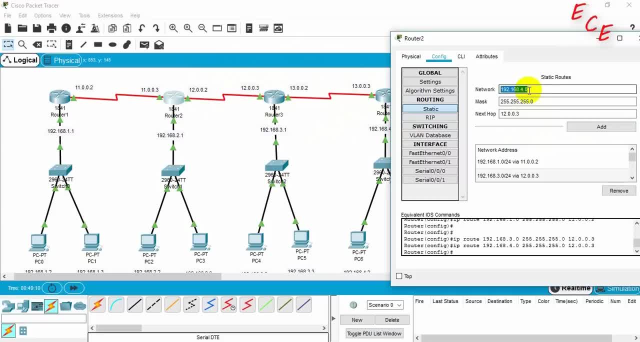 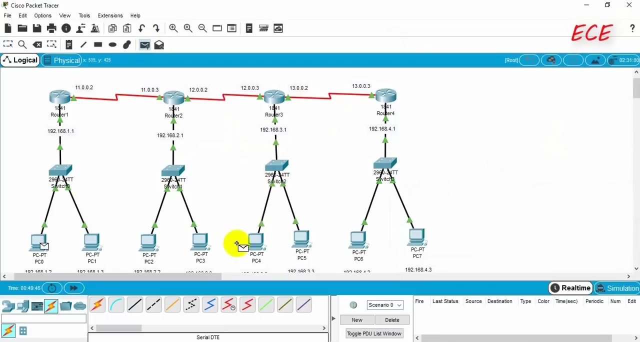 jump over one route to another, and now we need to connect the route with each other, because we are using a different route to access another. so here we will access route 13 with the help of route 12. now, if we want to send data, you can see that this will go back there. 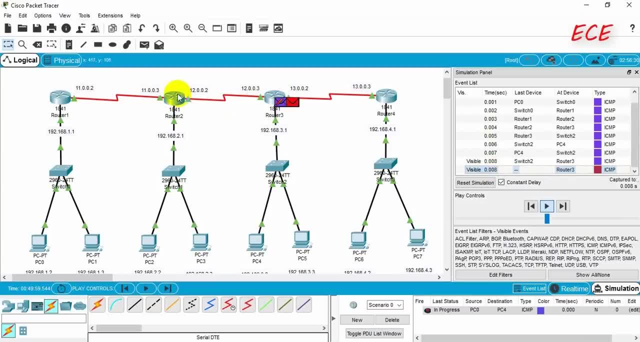 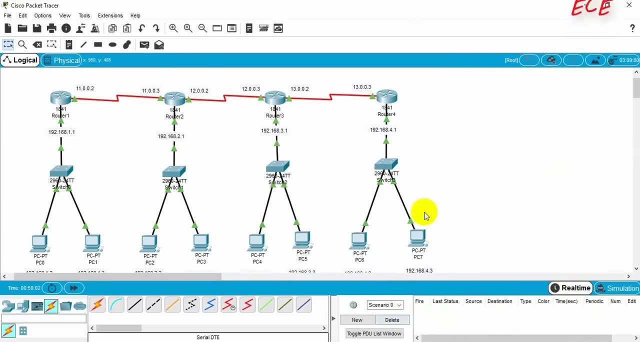 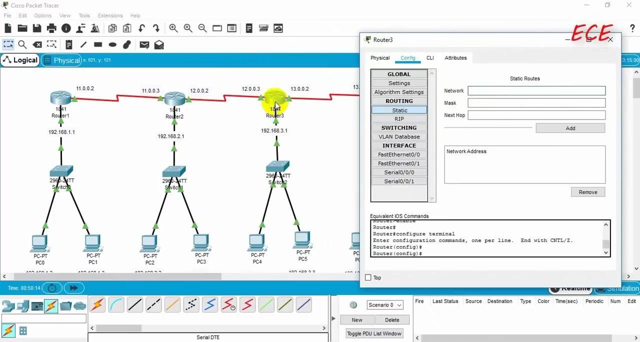 but you can see that it cannot go back because we have not configured the third router yet. so from the third one we need to send back to second router. so let's write it also. we need to send it to the first router too. so first let's do this 2.0 and 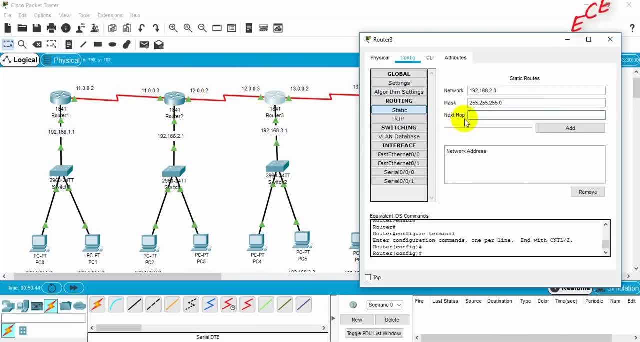 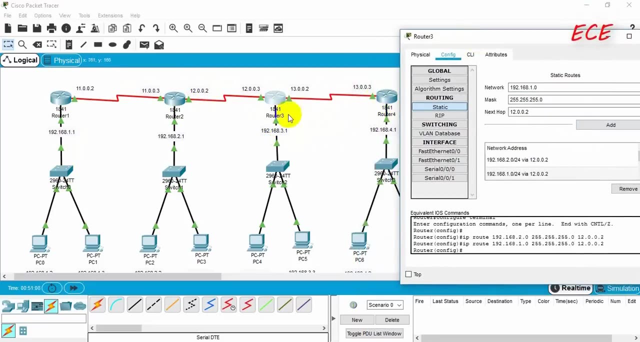 we will access it through the second routers IP address that is 12.0.0.2, and add it. then we need to send it to first one, so 1.0. the next hop will be same again. we cannot access it by jumping over one router. so after this we 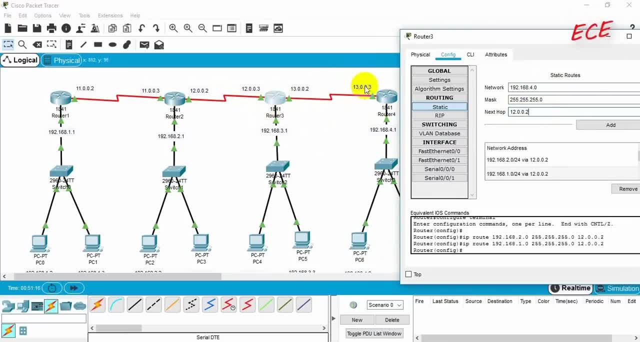 need to send it to router 4, so 4.0 and this one. the next hop will be router 4's IP address. okay, now we cannot send the data from the third router to first one directly, so we need to access that route 11.0.0. the mask will be 255.0.0.0 and here the next hop will. change to 12.0.0.0.2, then now we need to configure router 4. from router 4 we need to send back data to 3, 2 & 1 Y. at the last one, the first router is connected to the ro generu. 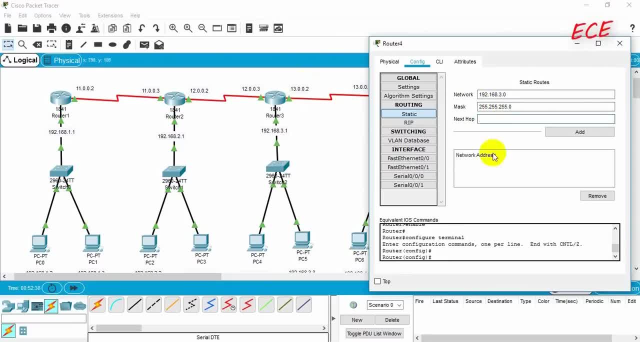 directto W route it normally to the same can be using. this is ayan. third routers next up and now to 4 to the next up will be same and for one, the next up again will be same. now we need to change the route, we need to connect. between the roots. so connect the roots already. so le take the path you will be. paste the top now. so connect the�든 r crap your port end. now connect to the laptop. let's continue. we have click below to ever debate. we are done. now we leave my. 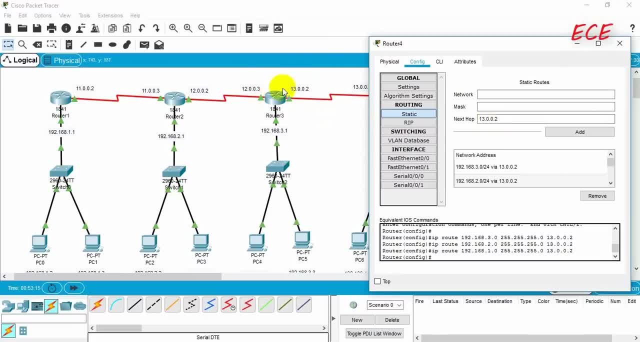 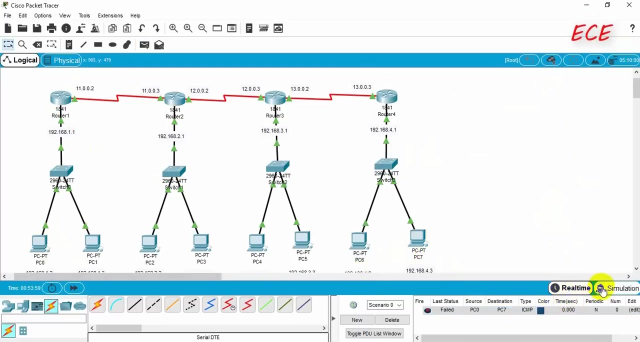 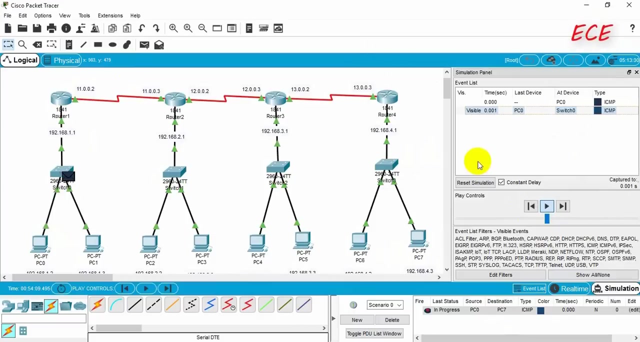 So route 12 will be accessed via this route 13.. And let's say route 11 will be connected via route 12.. Now if we send from PC0 to PC7, you will see that process will work properly. The data will be sent and the signal will send back, a signal to let the PC0 to know. 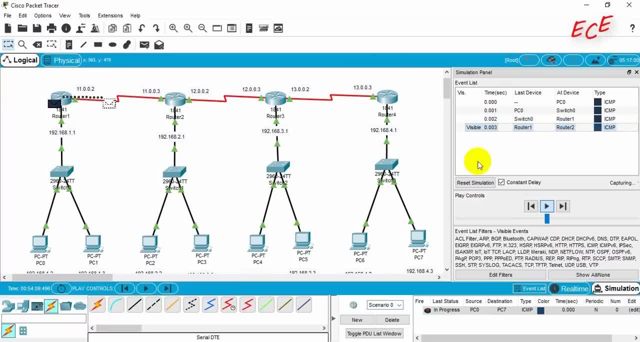 that it has received the data. We can send data from any PC to any PC in this network. Let's send from this one to this one, Okay, PC3 to PC4.. Sometimes it can fail the first time you send a message. 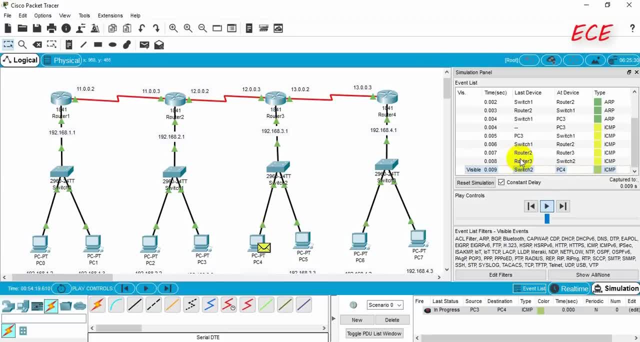 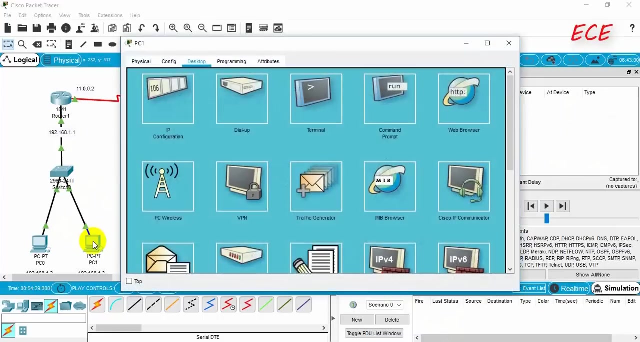 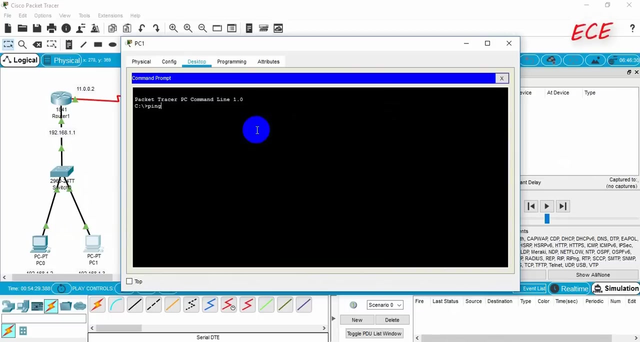 So try it for the second time again. We can also ping from one PC to another PC to know how it is working. Okay, Go to command prompt and write ping and then any of the IP address from any of the network. The first time you ping it will take some time.